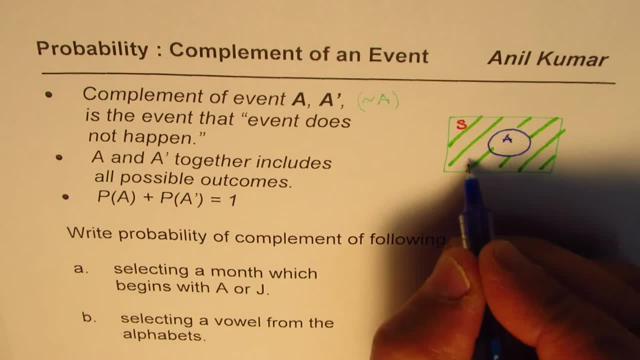 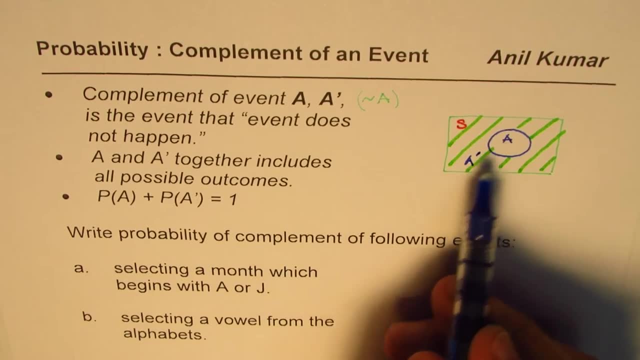 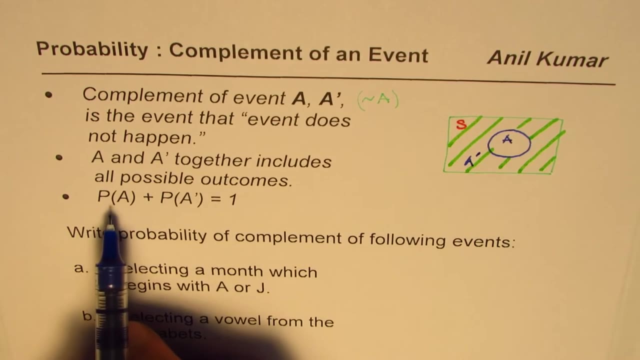 as complement of A. So all this is A prime complement of A. So you can see here that complement of an A and A totally is equal to the whole thing, right? All the outcomes possible and therefore probability of sum of event A and its complement will always. 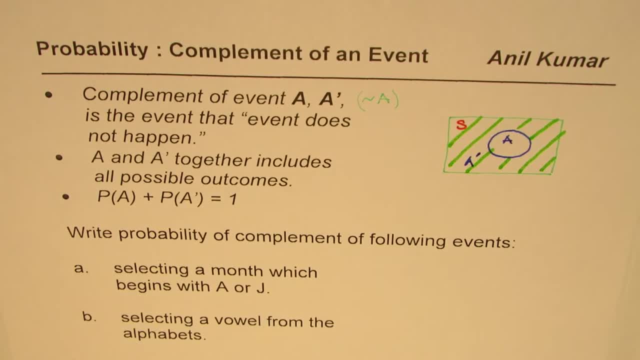 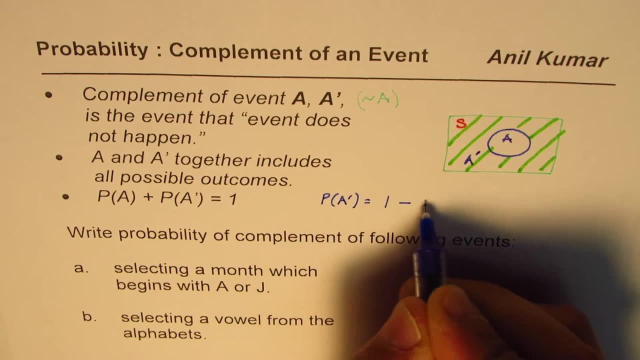 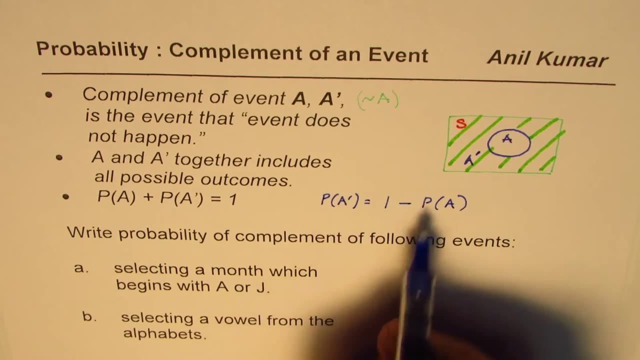 be A. So that is very important to understand. So from here you can also write that the probability of complement will be one minus probability of the event, right? So we can sometimes use this equation to find probability of complement. So the question here for your reference is: write probability of complement of following: 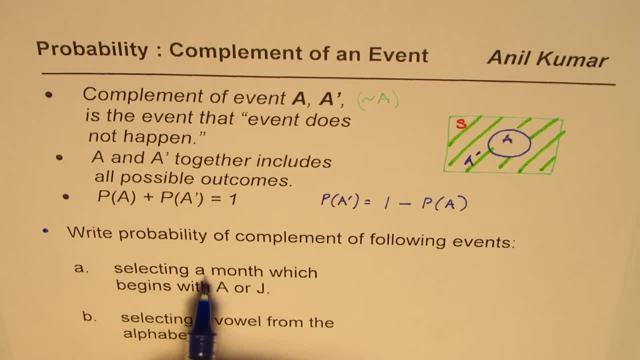 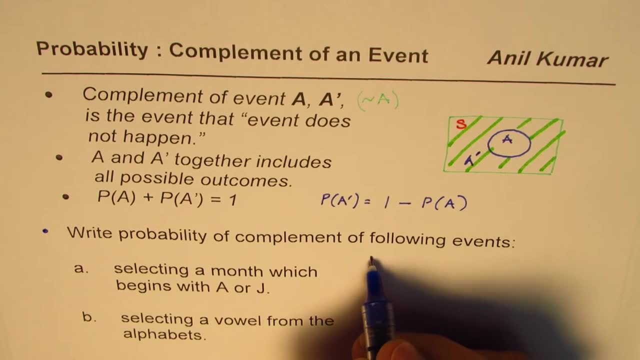 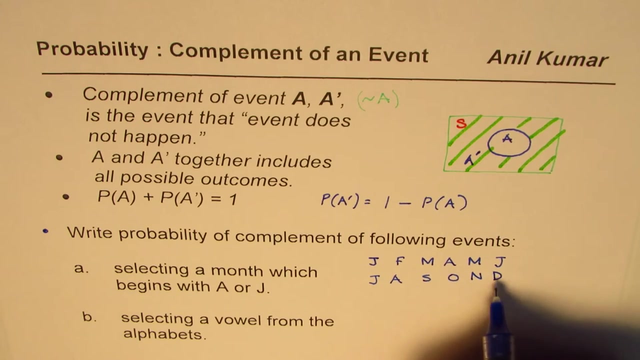 events. So we have selected two events, Selecting a month which begins with A right. So we have into the months we have, January, February, March, April, May, June, July, August, September, October, November and December. So we have 12 months in all. Now, if I want to say probability, 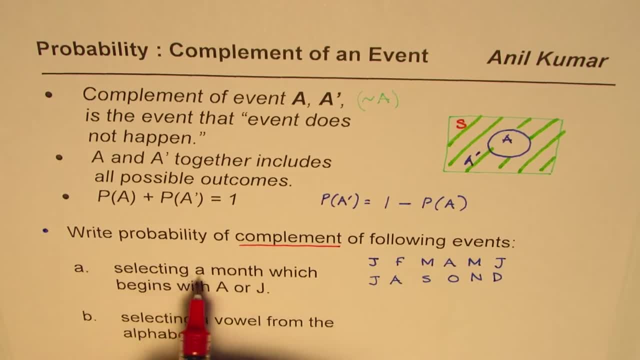 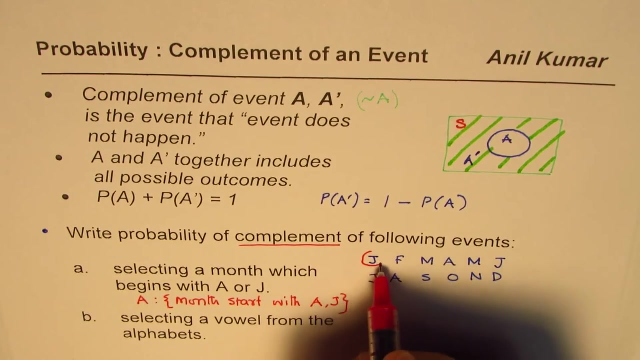 of complement of these right, So do not write probability of months which start with A or j, complement of this right. so so let us say event a is is month start with a or j right, so union of these two. so we can circle these months. so these are the months which start with a or j right. 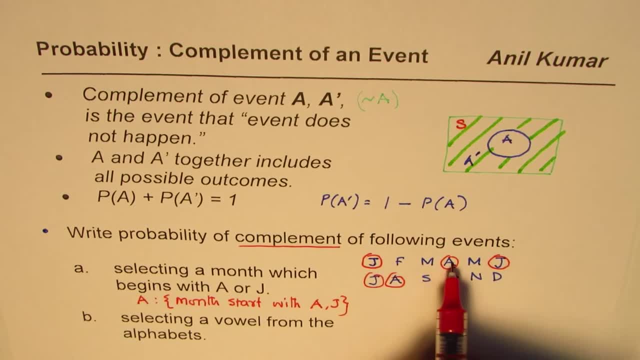 so these are the months one, two, three, four, five. right then, what is complement of a complement is months not starting from right, not start with letter a or j, do you understand? so that is what is complement. so we need to find probability of this. so there are two ways to go about.